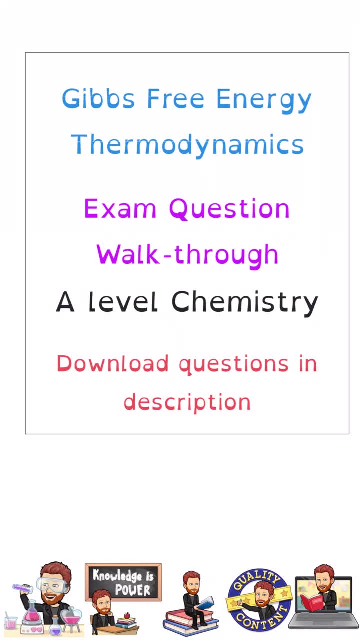 Hello and welcome to this A-Level Chemistry exam question walkthrough video where I'm focusing on a Gibbs free energy question from the thermodynamics topic. Have a go at this question yourself by downloading it from the description. then watch this video and see how you got on Throughout. 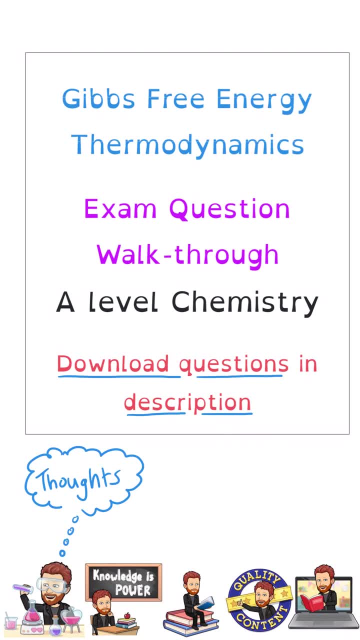 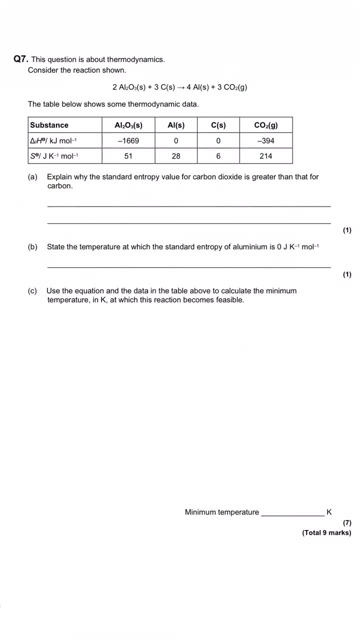 this video. I'll be modelling my thinking and writing that down in blue, and the answers that are going to get you the actual marks will be written in purple. This question is about thermodynamics. Consider the reaction shown. We've got two moles of aluminium oxide, which is a solid 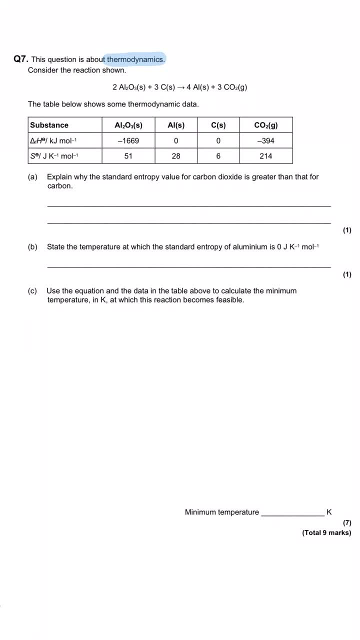 reacting with three moles of carbon, also a solid, and it turns into four moles of aluminium- still a solid- and three moles of carbon dioxide- this time that is a gas, and we've been given some thermodynamic data here for our four substances along the top row, We've been given enthalpy. 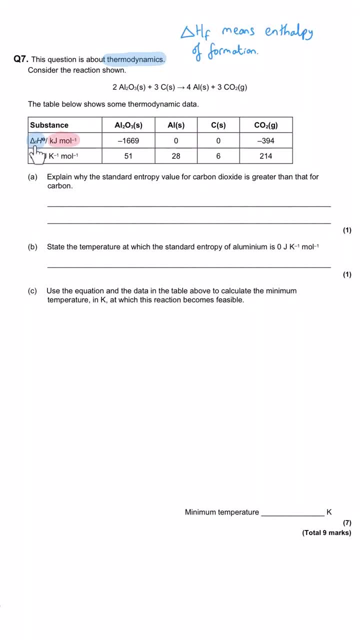 change values in kilojoules per mole And the enthalpy change values are enthalpy of formation. You can tell that from the little subscript here. As a result of it being enthalpy of formation, we can see that we've got two zero values. 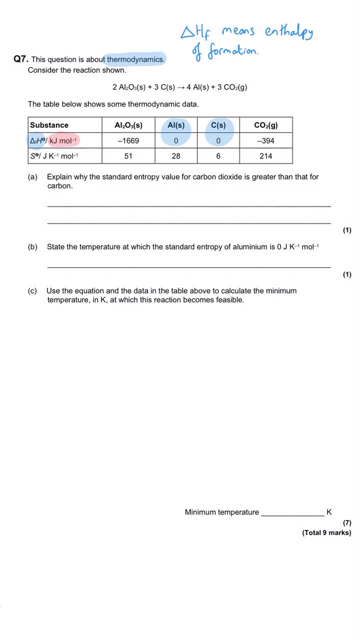 for aluminium and carbon. Those are our two elements. By definition, the enthalpy of formation for an element is zero, because the enthalpy of formation is when you, when you make a mole of something from its elements. So we can take a mole of carbon from a mole of carbon and expect that to have any enthalpy. 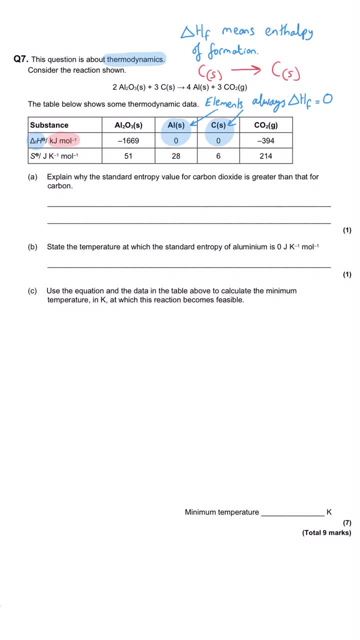 change, because we aren't actually changing anything. And so that's the same for aluminium. The enthalpy change for formation for elements is zero. And then on the bottom row we've got entropy change, and that's in joules per kelvin per mole. And the fact that we've got 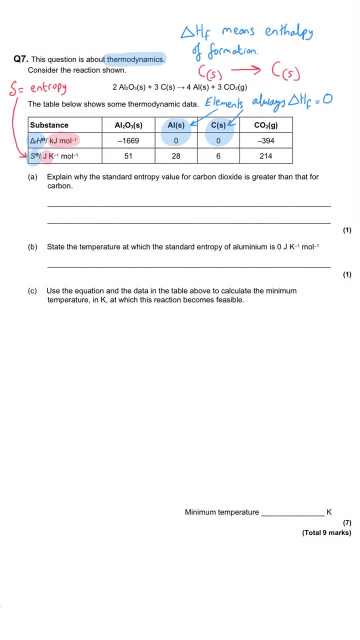 joules and kilojoules is going to cause us a problem that we're going to need to solve later. Part A says: explain why these numbers are independent. The answer is simple: The standard entropy value for carbon dioxide is greater than that for carbon. This comes down to the state symbols. Entropy is almost synonymous with disorder. 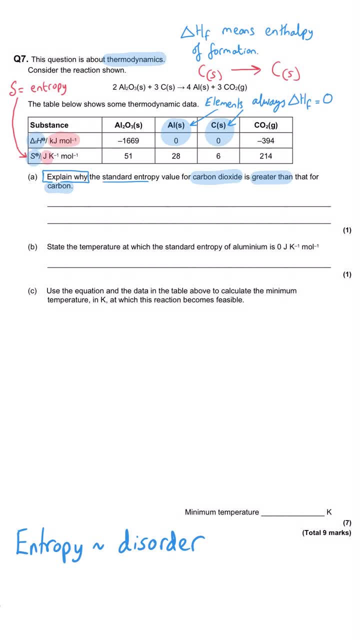 Not quite, but you can think of it like that. And so the more disordered something is, the more entropy it will have, And so a solid, which is what carbon is, is going to have much less disorder and so much less entropy than a solid. 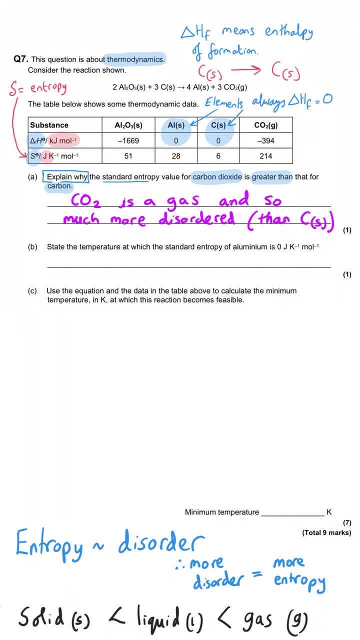 So the standard entropy value for carbon dioxide is greater than that for carbon, And so a solid carbon dioxide gas, or any gas, and so what you would need to say here is quite simply that carbon dioxide is a gas which is more disordered. Then part b says: state the temperature. 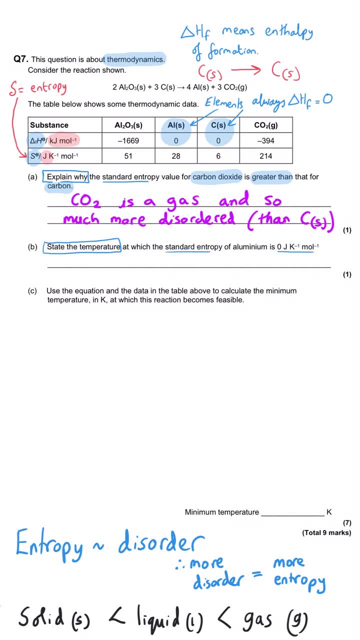 at which the standard entropy of aluminium is zero joules per kelvin per mole. Well, the fact that they're asking about aluminium is actually a little bit of a decoy here, because the temperature at which aluminium has an entropy of zero is the same for literally every substance in the world. 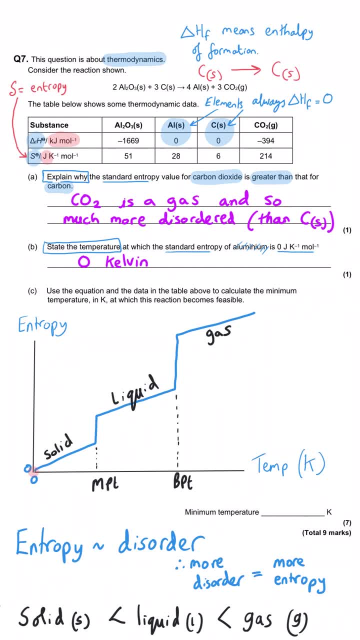 By definition, the entropy of any substance will be zero at absolute zero temperature, In other words, zero kelvin or minus 273 degrees c, because, by definition, at this temperature all of the particles will be absolutely stationary, not even vibrating a tiny bit. There is no movement of these particles and so there is no disorder, and so the entropy is set. 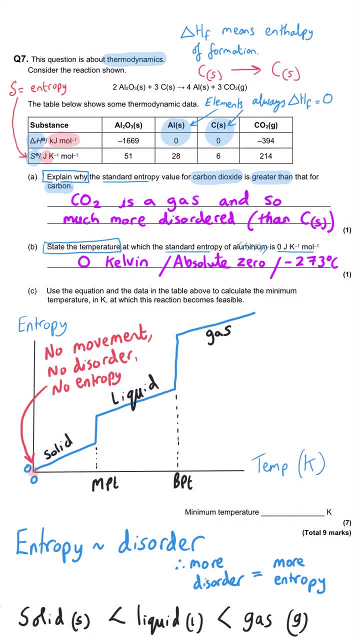 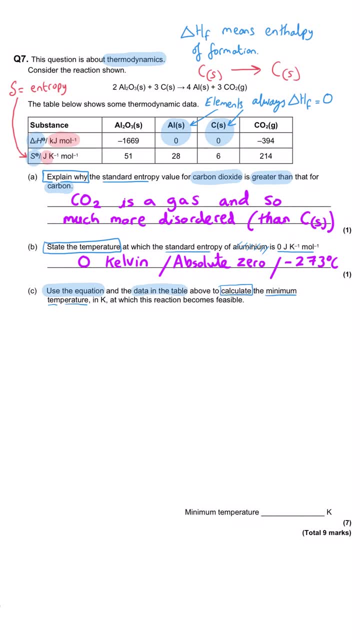 at zero, by definition, at this temperature. Part c says: use the equation and the data in the table to calculate the minimum temperature in kelvin at which this reaction becomes feasible. and so this is a seven mark question. so there's going to be quite a few different things to do here. 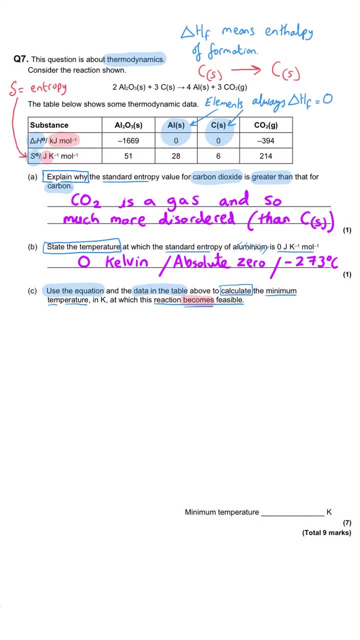 So feasibility is obtained from the equation for gibbs: free energy, which has got delta G, is equal to delta h minus T, delta S, and so this free energy, if it is less than or equal to zero, the reaction is going to be a feasible reaction. and then 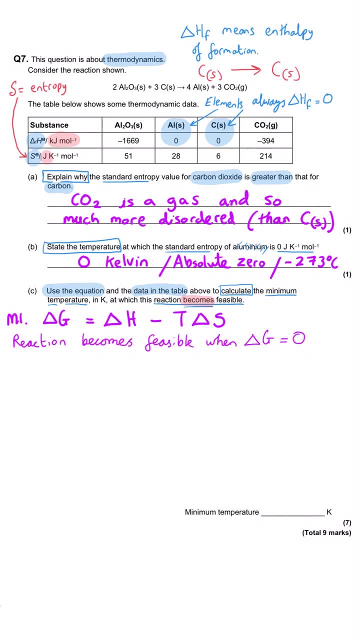 the reaction becomes feasible when delta G is equal to zero, And so what we get for our expression then is delta G Delta H minus T. delta S rearranges to when delta G is zero. zero equals delta H minus T delta S, So delta H equals T delta S, and so delta H divided by delta S is equal to the temperature T in Kelvin. 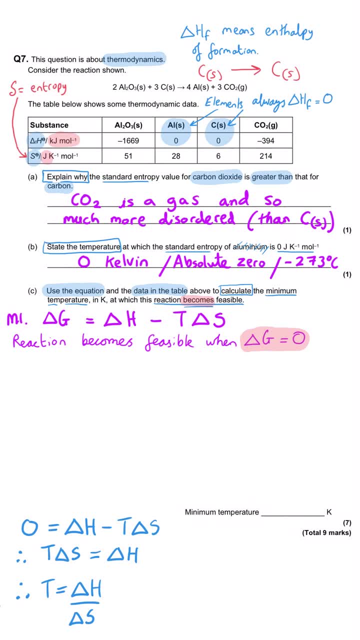 And so it's clear now what we need to do next. We need to calculate the temperature as our final answer. so to do that, we need to work out delta H, which is, of course, the enthalpy change for this reaction, and delta S, which is the entropy change. 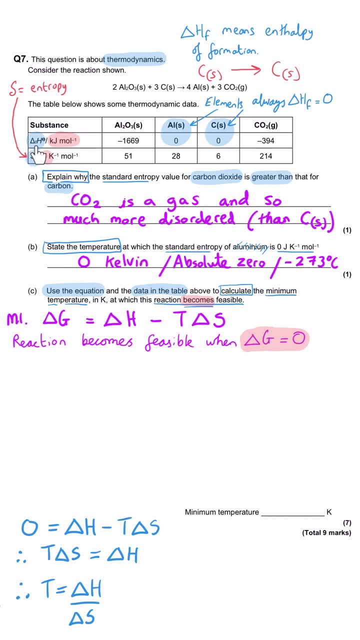 Now, because we're using enthalpy of formation data. the enthalpy change for this reaction is the sum of the enthalpy of formation of the products minus the sum of the enthalpy of formation of the reactants, And so what we need to do here, then, is look at our products. 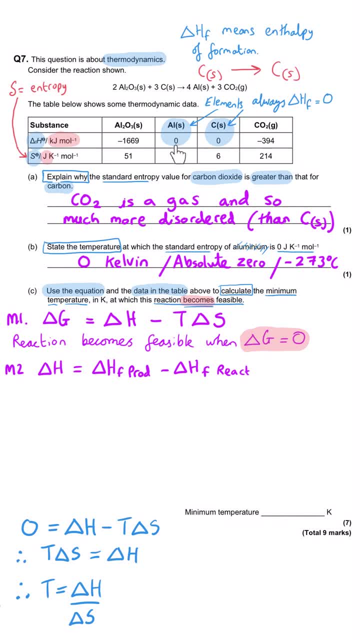 We've got four aluminium, Remember we've already said that the element is going to have. We have an enthalpy change of zero, so we can basically ignore that. but carbon dioxide is minus 394 kilojoules per mole and so we need to triple that because of the coefficients in the expression. 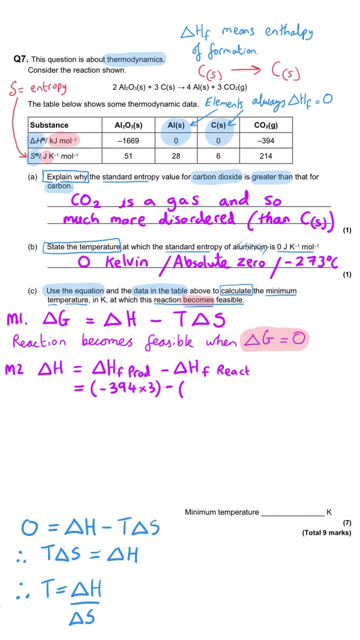 And then we're subtracting from that the enthalpy of formation of the reactants. Again carbon, the element is zero. so we're just looking at the minus 1669 from aluminium oxide, but again multiplying it by this coefficient of two. 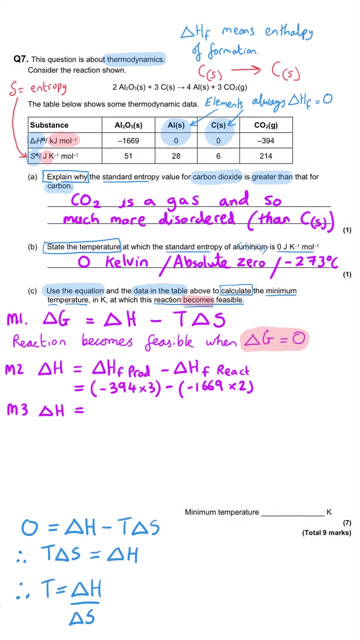 Once we crunch these numbers, the enthalpy change for this reaction comes out to be 2,156 kilojoules per mole, So an endothermic reaction. And then, when we look at the entropy change, entropy change is calculated in the same way that we use enthalpy of formation. actually, 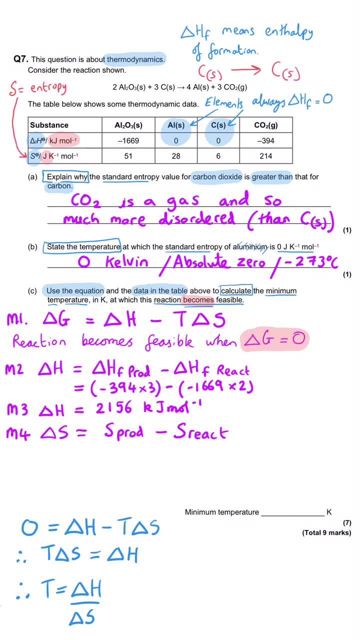 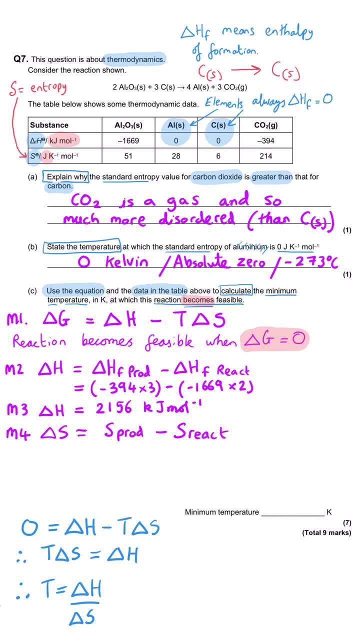 The entropy of the products minus the entropy of the reactants. And this is a little bit of a longer calculation because we don't have any zero values. So we need to take the aluminiums 28 and multiply it by four, add it to the 214 for carbon dioxide multiplied by three. 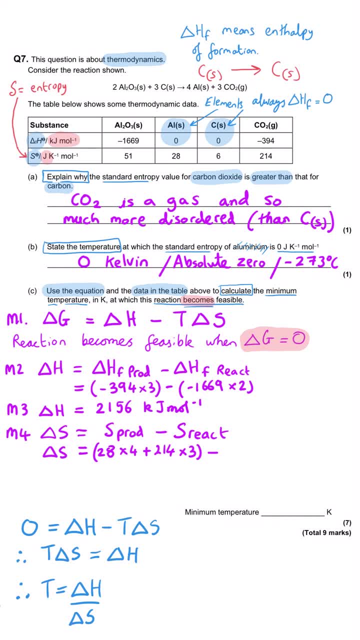 That is the sum of the entropy of our products, And the sum of the entropy of the reactants is two multiplied by 51, and then six multiplied by three, And when we calculate that that we get an entropy change of 634 joules per Kelvin per mole, So definitely an increase in. 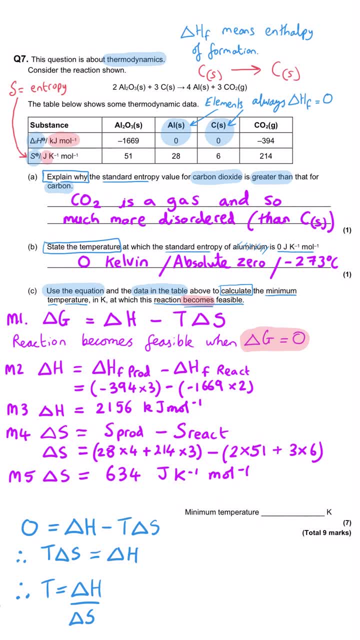 entropy as this reaction happens. Now we've got these two numbers, The temptation would be to put these numbers straight into the delta G expression. But we must do one extra thing before doing that, because enthalpy is in kilojoules per mole and entropy is in joules per Kelvin per mole, So we 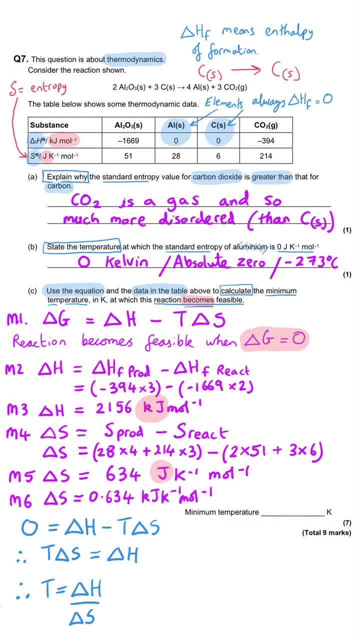 need to divide our entropy change by 1000 to get them both into kilojoules, And so 634 divided by 1000 is 0.634 kilojoules per Kelvin per mole. And then, last of all, we need to calculate our 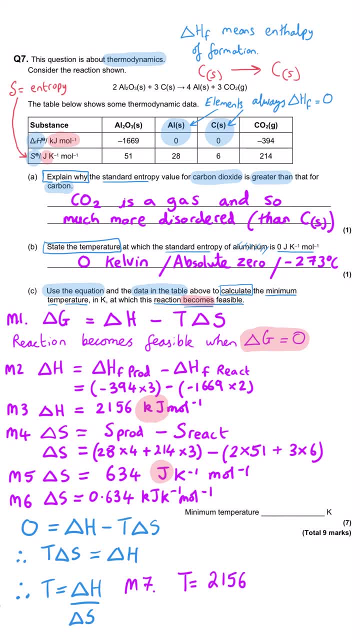 temperature. So we can put in our enthalpy change exactly as it was: 2156 kilojoules per mole divided by our entropy, now in kilojoules per Kelvin per mole of 0.634.. And we get a final answer to two significant figures of 3400 or it. 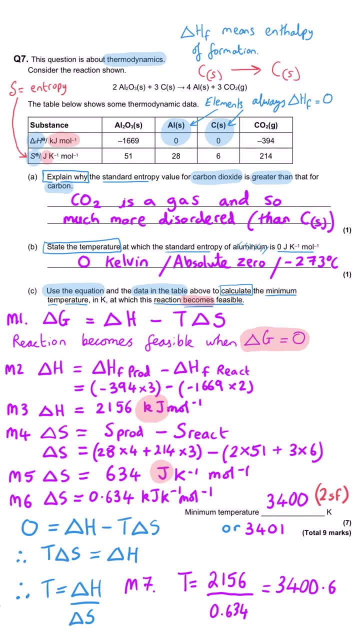 comes out to maybe 3401 Kelvin for a little bit more accuracy. And that's what we need to do for our seven marks. Each of these steps will get us one mark each And we will get transferred error if we make a mistake partway along Or, for instance, if we forget to divide our answer by 1000,. 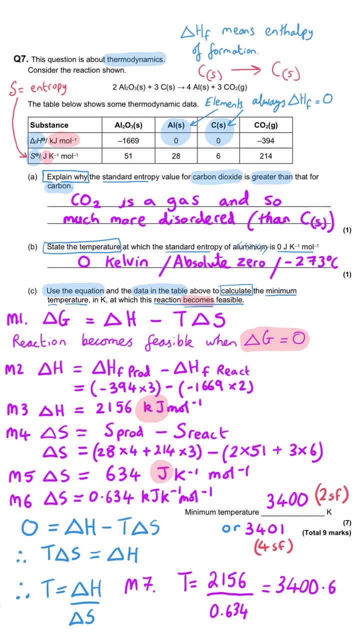 we would lose the penultimate mark but probably get the final mark, And it's really important, therefore, when we're looking for method marks, to structure our calculation clearly so the examiner can see what we've done and can give us method marks if we don't get that final answer.